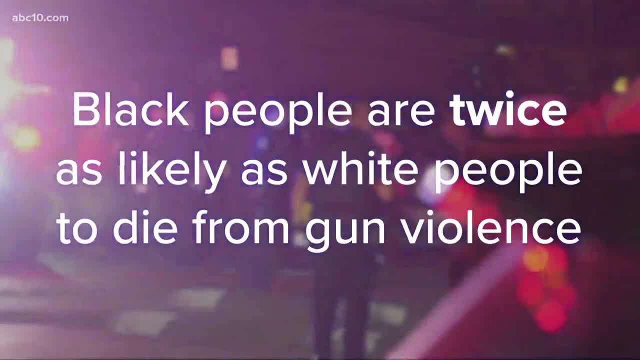 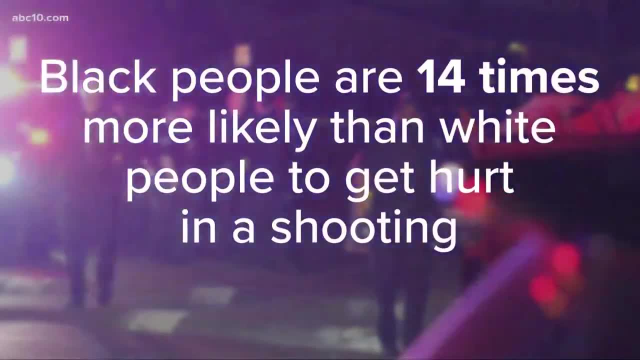 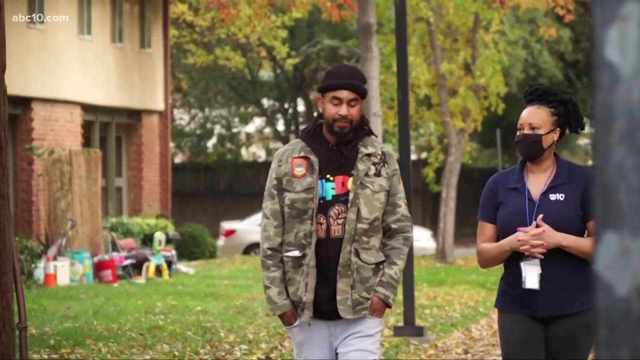 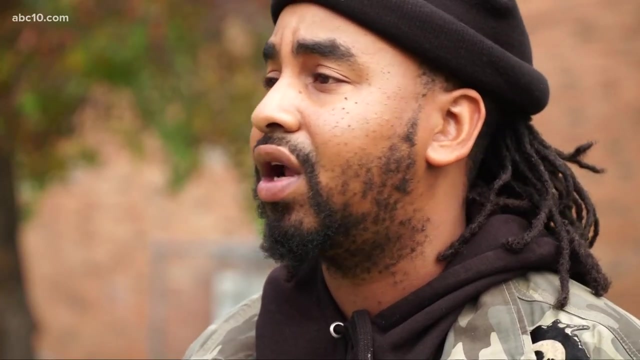 twice as likely as white people to die from gun violence. That's coming from the CDC and data collected by the Giffords Law Center to prevent gun violence. It shows black people are also 14 times more likely than white people to get hurt in a shooting. The Black Child Legacy campaign is a nonprofit in Sacramento working to change those alarming statistics. We have programs that have been in this community all over Sacramento- you know the last 30 years- but we're not able to serve. 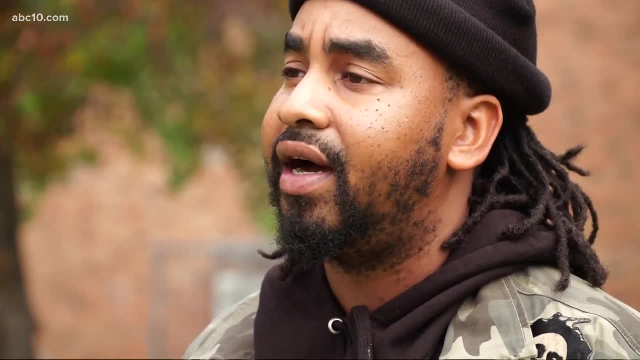 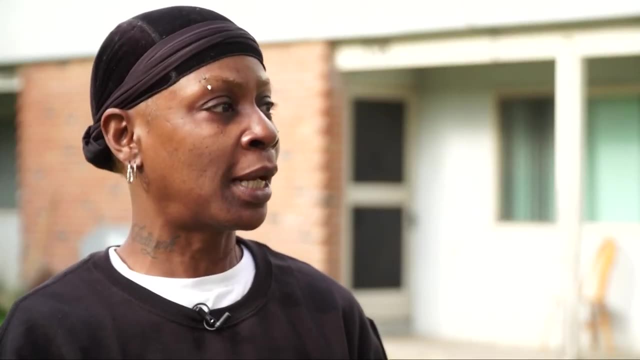 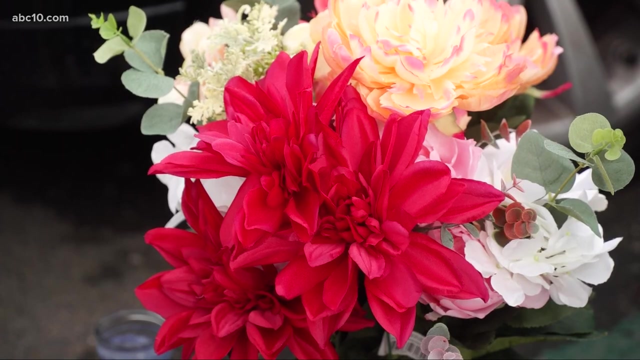 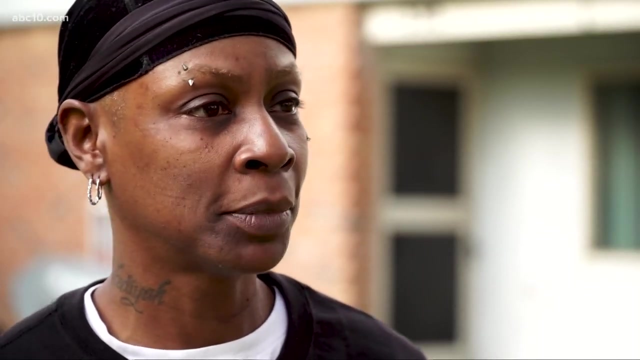 the way we would like to by being underfunded. Kenneth Duncan, with the group, says they need more funding for intervention and gun violence prevention programs. I'm pondering, like, what can I do as somebody in society, as an adult? Cammie Wilson, who lives in an upper land park housing complex, says gun violence is not unheard of in the predominantly black and brown community. Oh no, Oh no, It's not even unheard of me growing up, And that's what's sad. We see more deaths sometimes than men who've been in the community. 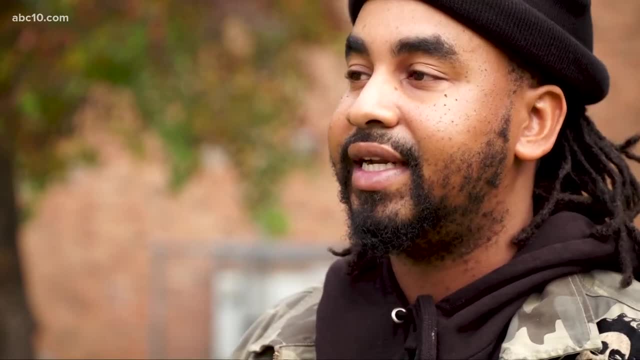 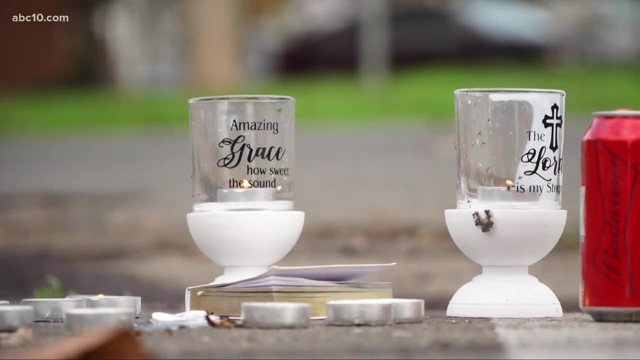 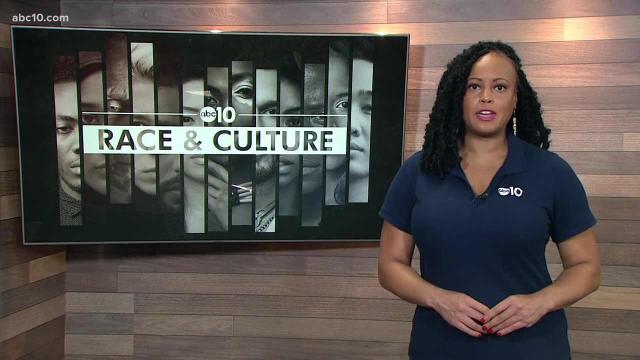 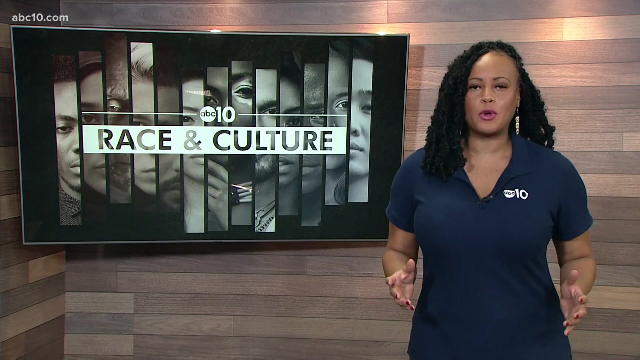 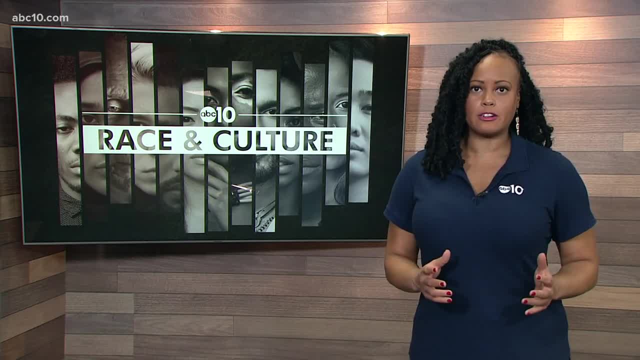 SORTS OF ORGANIZATIONS ARE LOOKING FOR MORE FUNDING, VOLUNTEERS AND SUPPORT OVERALL. CHRIS, SOMETHING NEEDS TO BE DONE. IT CERTAINLY GETS YOUR ATTENTION WHEN SHE TALKS ABOUT THESE EXPERIENCES ARE ALMOST LIKE. 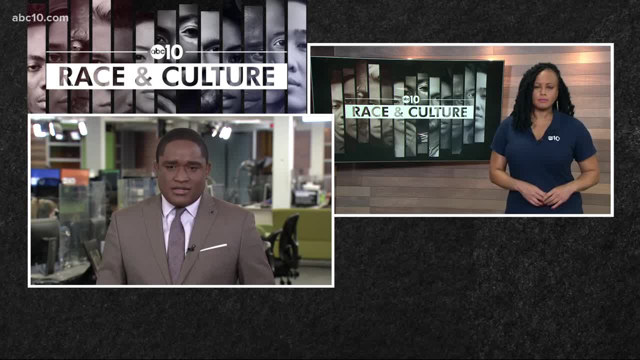 FOLKS ARE IN A WAR ZONE WITH SOME OF THE THINGS THEY'VE HAD TO DEAL WITH THROUGHOUT THE YEARS.